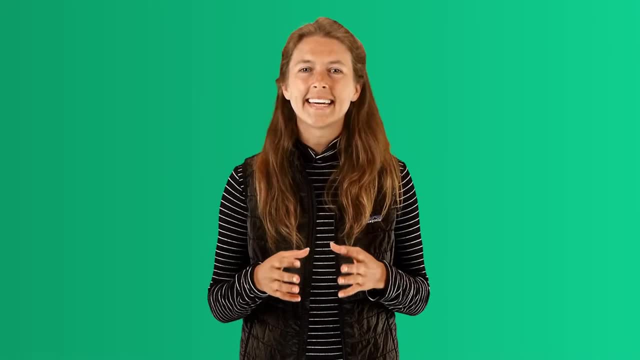 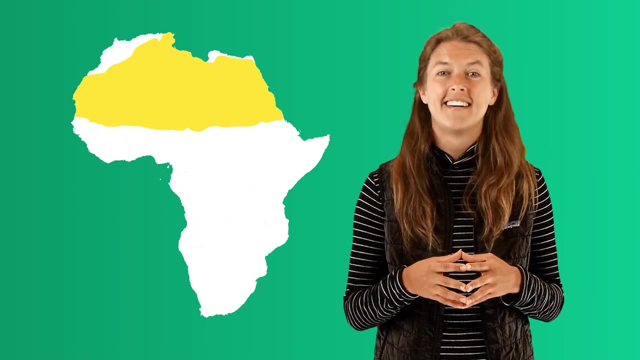 making it feel like summer all year round. It contains the world's largest desert, the Sahara, which is almost the size of the entire United States of America. Africa also contains one of the world's longest rivers, the Nile River in Egypt. 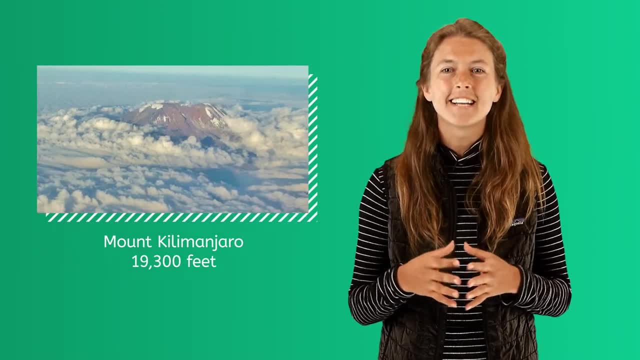 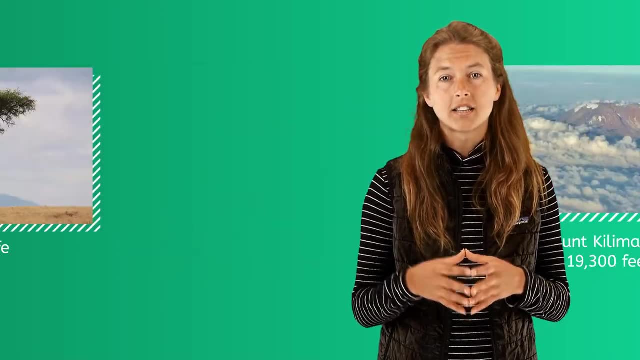 cutting through 11 countries. Mount Kilimanjaro is the highest mountain in Africa. Africa is home to some of the world's most amazing animals, like the tallest animal, the giraffe, the deadliest land mammal, the hippopotamus. 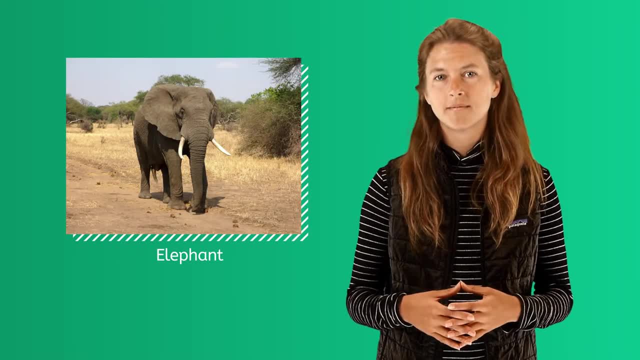 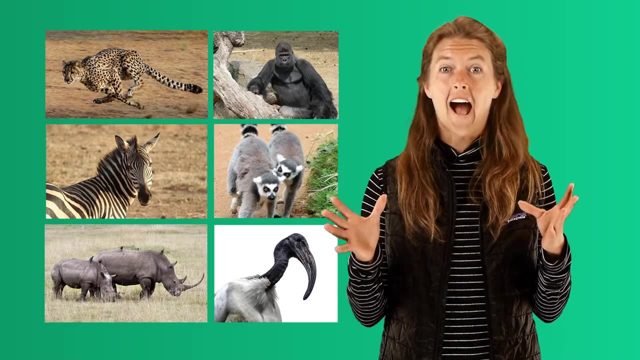 and the largest animal on land, the elephant. You can also find cheetahs, gorillas, zebras, rhinos, lemurs and many unique birds. Wow, Africa is the most multilingual continent in the whole world, where thousands of languages 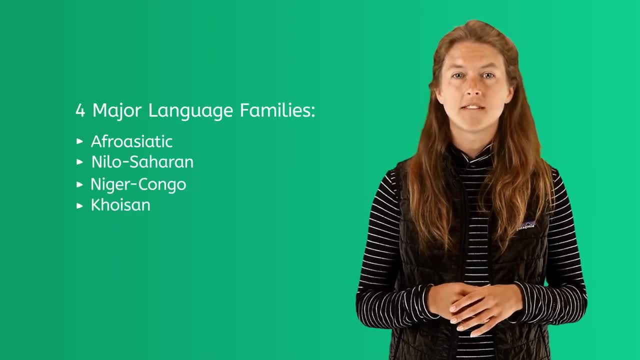 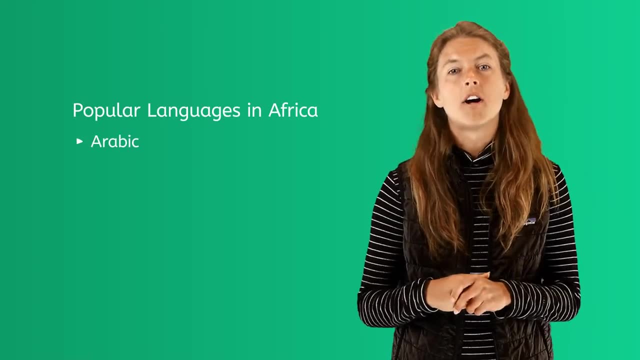 are spoken with four major language families native to this continent. Arabic is a popular language in Africa, followed by English, Swahili and Swahili. It is the most popular language in the world. The majority of the population of Africa are African-American and French. 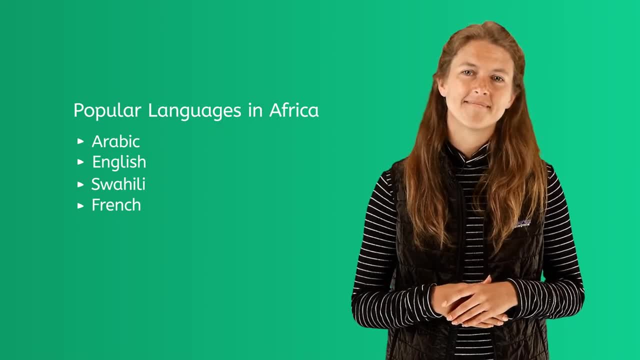 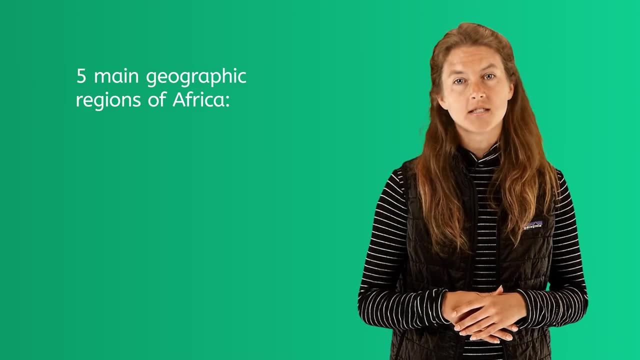 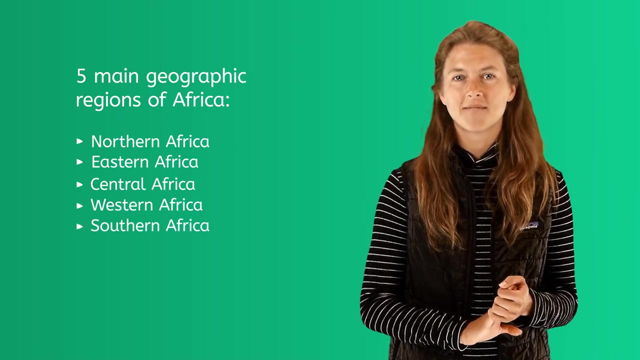 Interestingly, there are more French-speaking people in Africa than in France: There are 36,842 people. Africa is the continent with the most amount of countries in it- 54,- with five main geographic regions—Northern Africa, Eastern Africa, Central Africa, Western Africa and Southern. 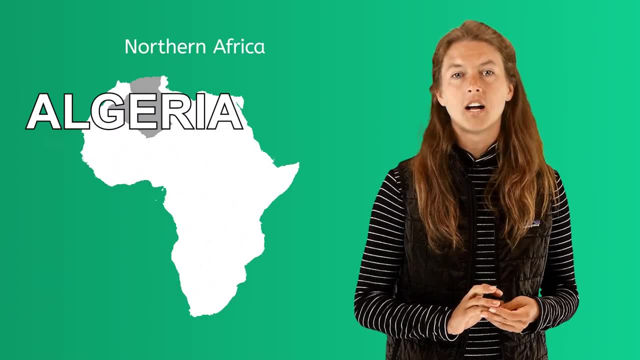 Africa. Let's look at the countries within each region. One of the countries within the African continent is North Africa. Two countries within the African continent is the Middle African region. One is northern Africa, The other is northern Africa, the largest country in Africa, and Egypt, which is a very popular tourist. 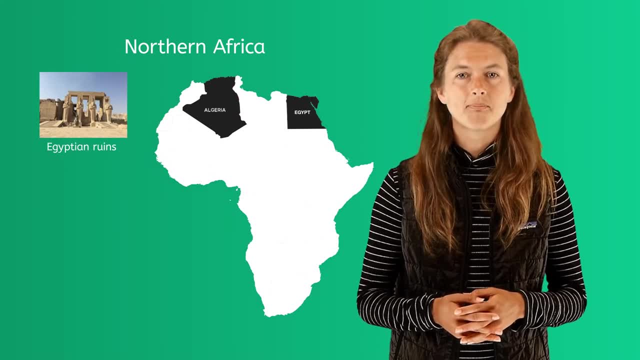 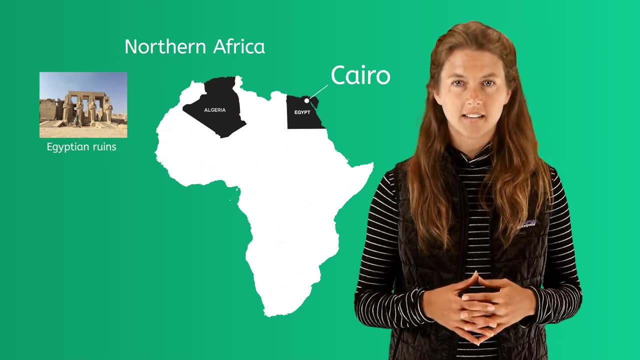 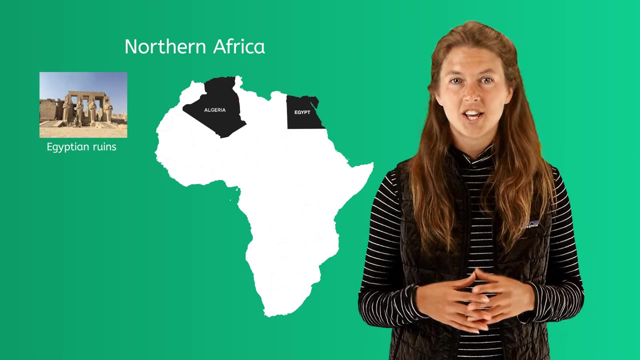 destination because of the Egyptian ruins. it also contains the capital city, Cairo, which is Africa's largest city. Egypt is home to one of the world's oldest civilizations, the pharaonic civilization. you have probably already heard about the ancient pyramids and temples found in Egypt. Egypt is a 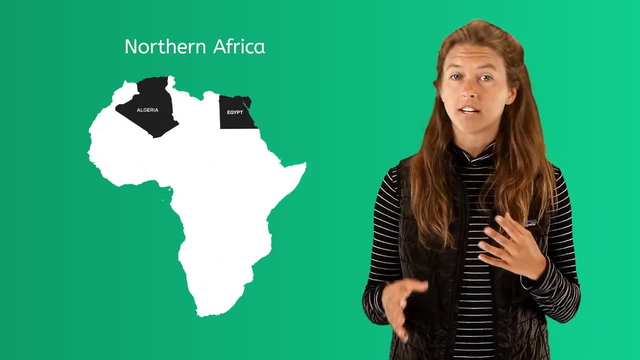 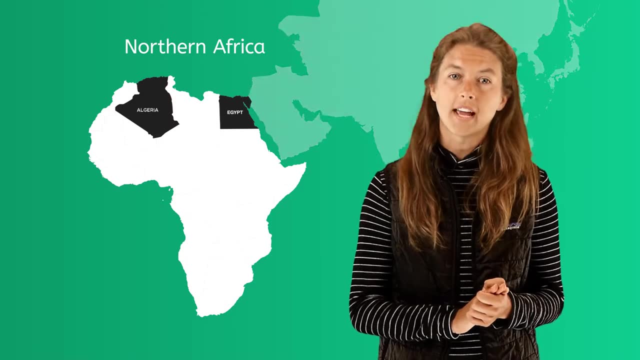 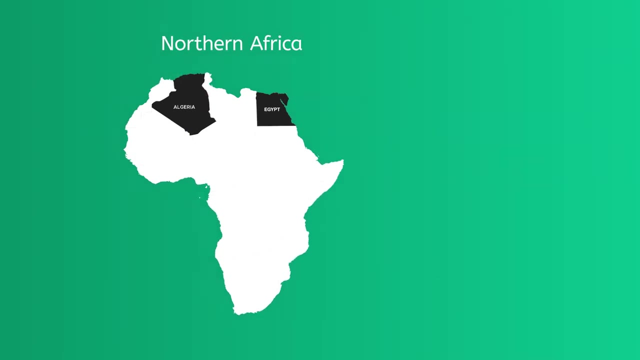 transcontinental country, which means it is part of different continents. Egypt itself occupies the northeast corner of Africa and also the southwest corner of Asia, which is also known as the Middle East. Wow, also in northern Africa, Libya, Morocco, which is the number one travel spot on the continent of Africa, Sudan and Tunisia, another popular travel spot. 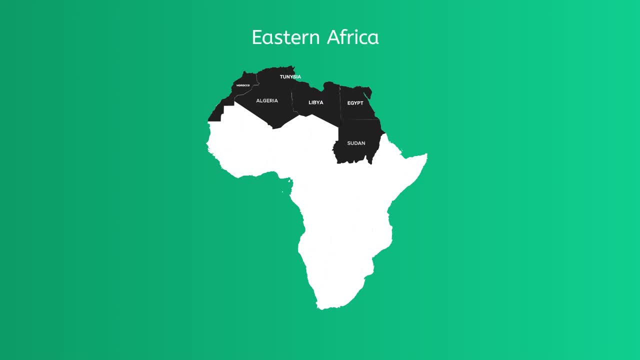 Egypt is home to the largest island in the world and is home to the largest. let's move on to eastern Africa. next we have Burundi, Camaros, Djibouti, Eritrea, Ethiopia, where the oldest human remains were found- Kenya, Madagascar, which is the 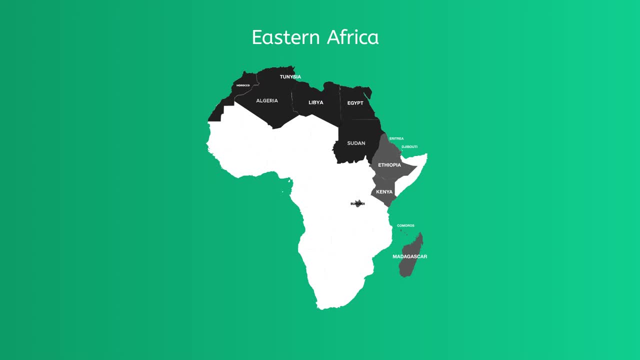 largest island in Africa and the fourth largest island in the entire world- Malawi, Mauritius, Mozambique, Rwanda and the Seychelles- which is a group of 115 awesome small islands, making it a popular beach destination. Continuing in this region: Somalia, South Sudan and Tanzania, home to the Serengeti, where 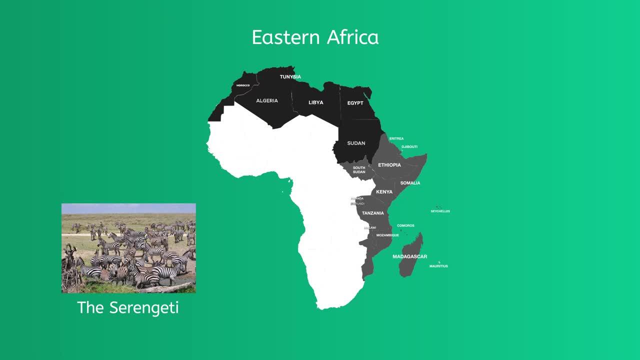 thousands of animals migrate or seasonally move to a new area. You've probably seen images of zebras impressively marching in large herds. Finally, in the eastern region of Africa, we have Uganda, Zambia and Zimbabwe, home to one of the world's seven natural wonders, Victoria Falls, which is the 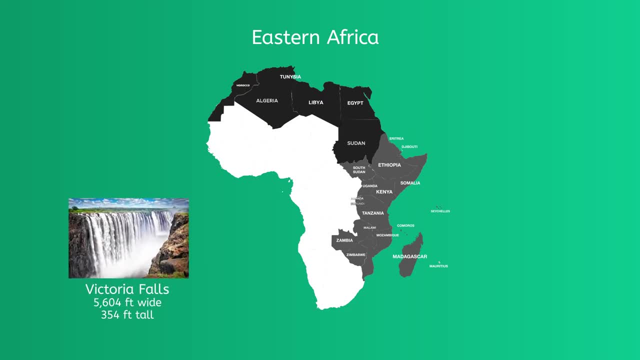 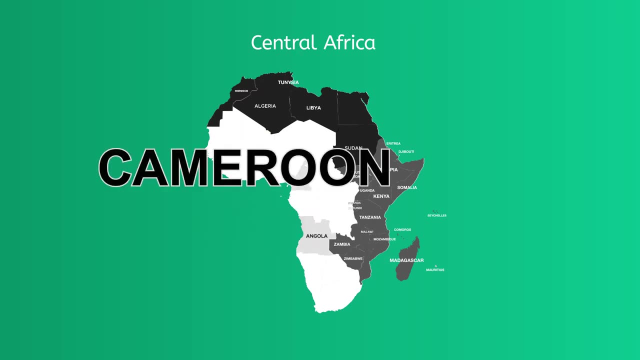 largest waterfall in the whole world. Let's travel to Central Africa now. Looking at the countries, we have Angola, Cameroon, the Central African Republic, Chad, the Democratic Republic of the Congo and the Republic of the Congo. Finally, you can find Equatorial Guinea. 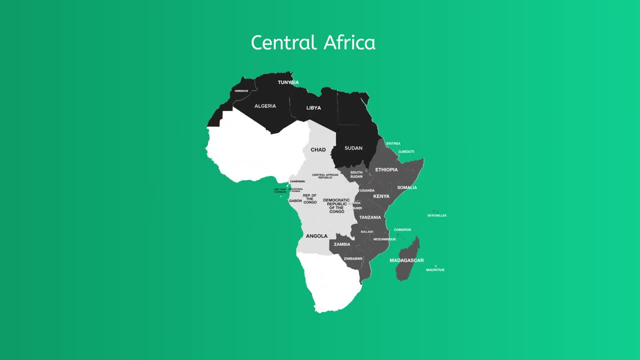 Gabon and Sao Tome and Principe. Okay, now for the countries in Western Africa: Benin, Burkina Faso, Cape Verde, Gambia, Ghana, Guinea, Guinea-Bissau, Ivory Coast, Liberia, Mali and Mauritania.